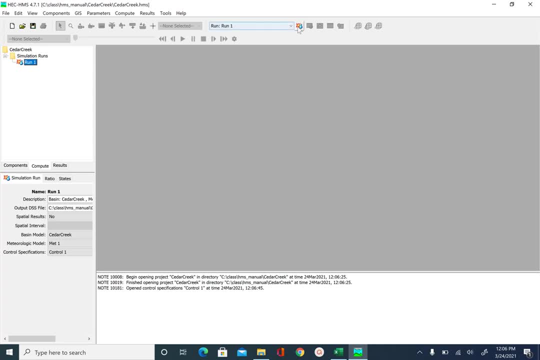 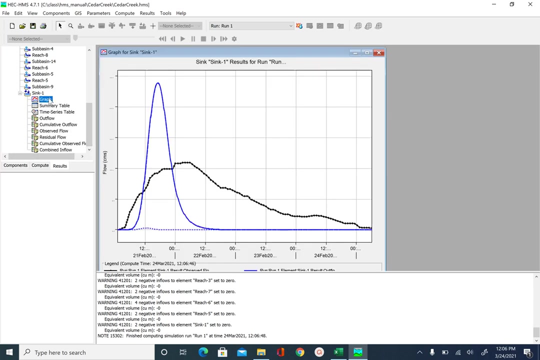 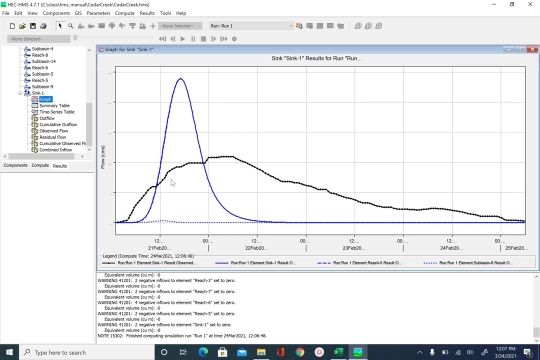 you can go to compute, pick run 1 and run the simulation with this button. So this is the simulation button, So close. And then you will go to sync, which is the outlet, and look at the graph. So you can see that the blue line is the model output and the black dots that you see. 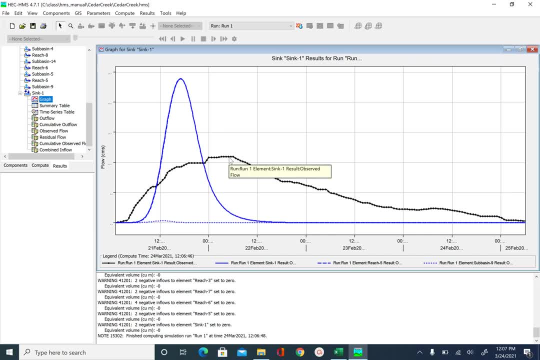 here is the observed hydrograph. So in calibration, what we try to do is we try to match this blue model output hydrograph with the observed hydrograph. So in order to calibrate the model, we should also know how some of the parameters impact the hydrograph shape. So, if you remember, we used the SCS. 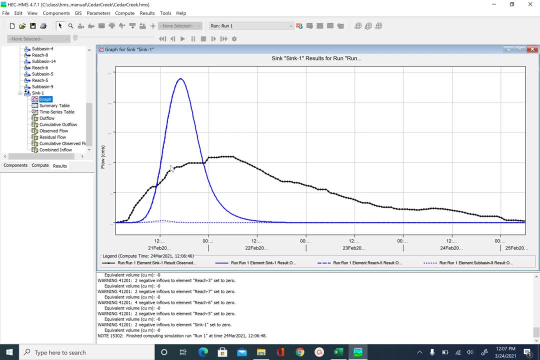 curve number method for computing loss and we use the SCS unit hydrograph method for transforming runoff into hydrograph and then we use the Muskingum method for routing. So you can see that our model peak is very high compared to the observed hydrograph and then we can see our peak is happening. 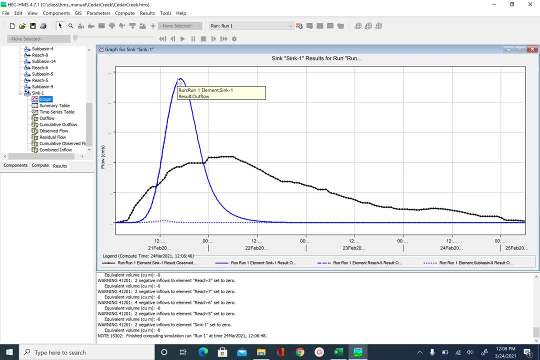 earlier than the observed peak. so we have to shift the peak, we also have to reduce the peak and then you can see there is a lot of volume difference between the observed hydrograph and the model hydrograph towards the tail end. so we can work to fix that too. so we know that the curve number affects the 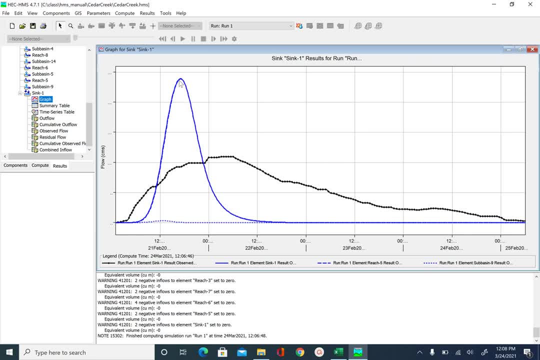 hydrograph peak. so one initial iteration you can do is you can reduce the curve number and see how this impacts the hydrograph shape. so in manual calibration you have to change everything manually. so what we are going to do is we are going to click on components, pick the basin model that we want to calibrate. 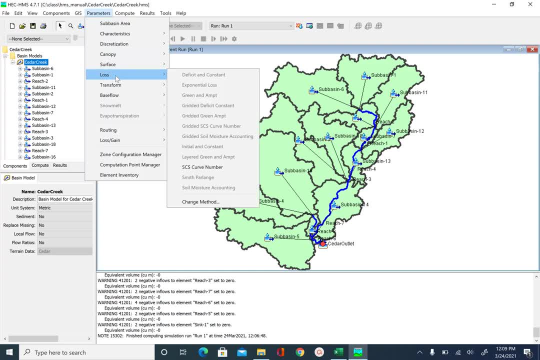 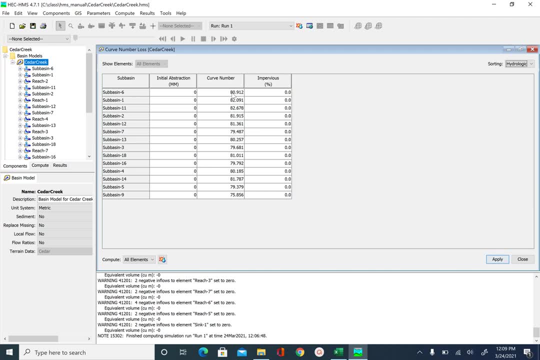 and then we are going to calibrate the hydrograph peak and then we are going to go to parameters, loss and SCS curve number. so this is our initial curve number that we use to create our first simulation. so what we are going to do is we are going to reduce this curve number to bring that peak down. so what you can. 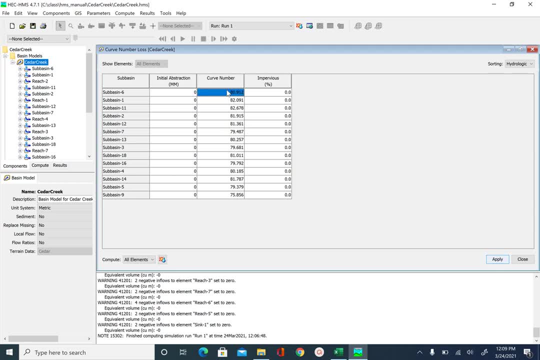 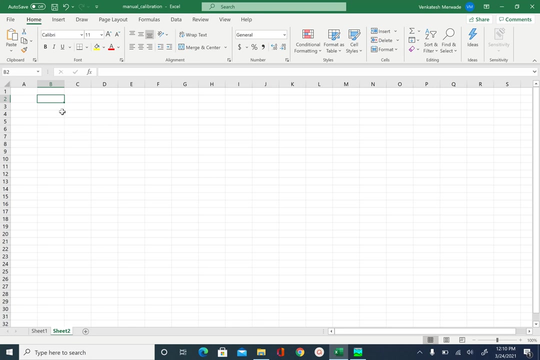 do in order to retain your original values. one way to do that is you can write this down manually somewhere or you can create an excel sheet. so I'm going to copy this. ctrl C or right click, copy and open an empty excel file. I named this file as manual calibration and here I'll. 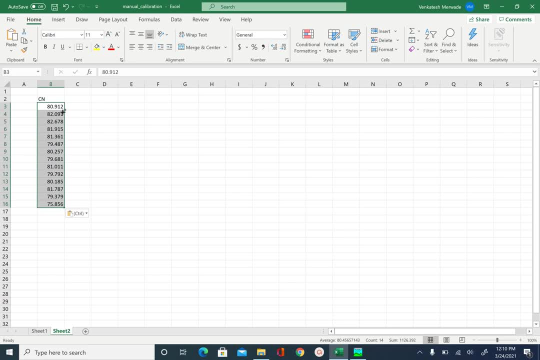 just create my curve number values. so this is my initial value. so, in order to bring this down, what I'm going to do is I'm just going to reduce it by 10%, so I can say 0.9% times the initial value, and then you just do that for all the sub basins and 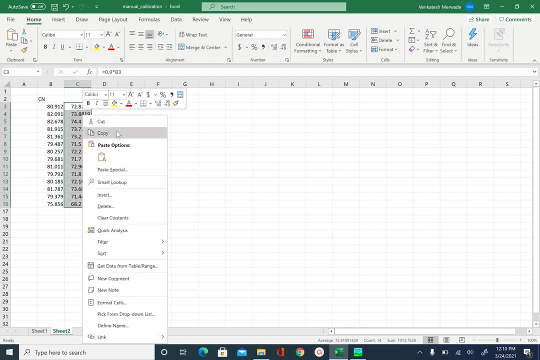 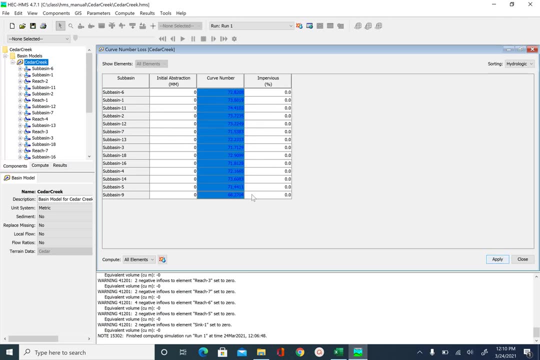 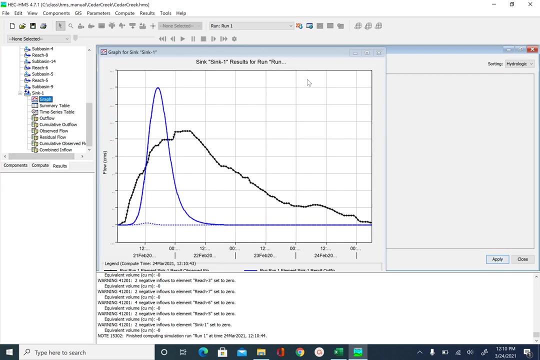 so I copy this now and then select ctrl, C or right click copy, go back and simply paste it here and then. and here we go, I paste this here and then I copy this and then run the simulation again and then we go. results: look at the graph so you can see that the peak did come down a little bit. 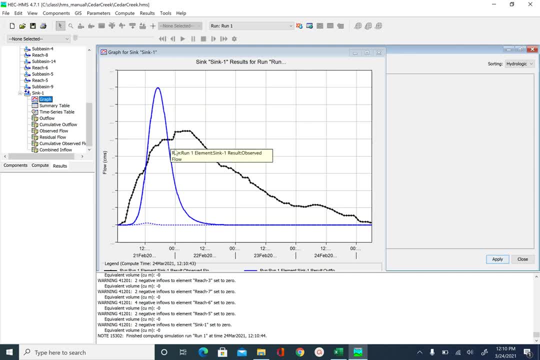 if you want, you can just play with curve number to bring this peak up to here. but we also know that lag time affects the peak in terms of the magnitude and also the position. so instead of just playing with the curve number, we can also try changing the lag time in order. 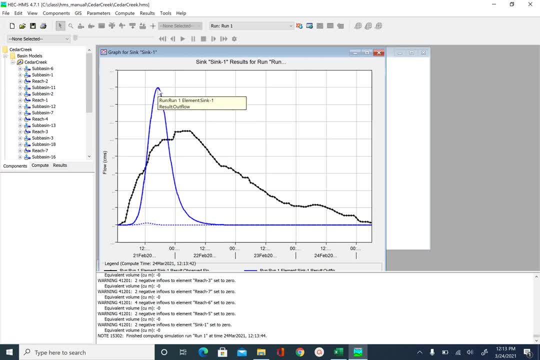 to bring this peak down and also shift this peak little later. so if we increase the lag time, the peak will go down and hopefully this will shift towards where the observed peak is. so in our next iteration let's go ahead and change the lag time. so to change the lag time you will go to components. 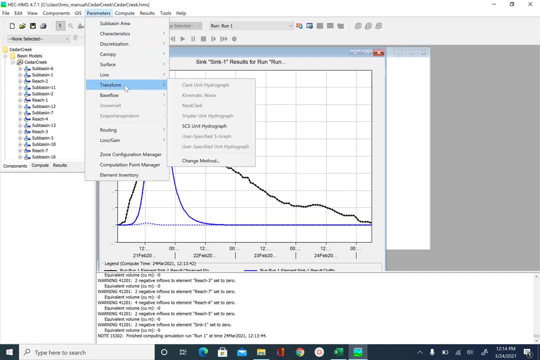 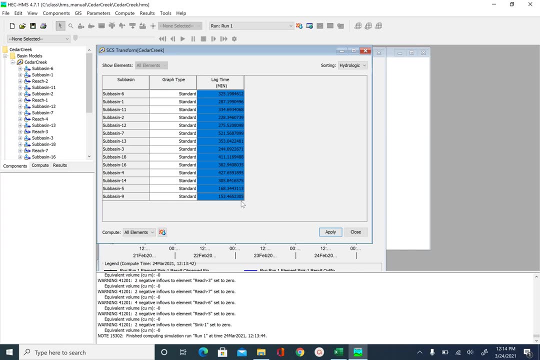 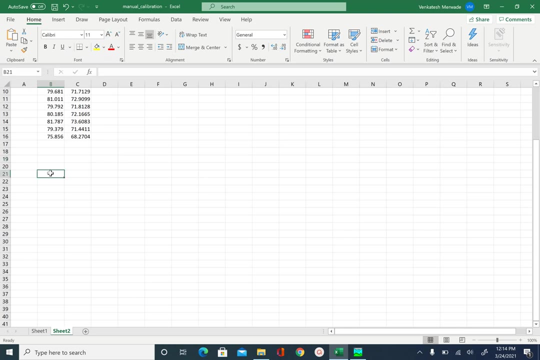 here for basin one: parameters: transform, scs, unit, hydrograph, and these are our initial values. so we will copy them, select, copy and then go to excel and we will create our lag time series here and paste. so we are going to increase the lag time for our second iteration, so let's increase by. 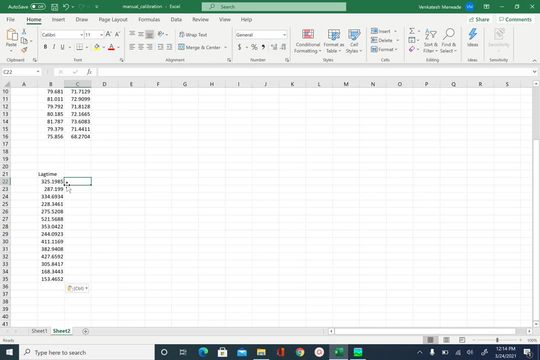 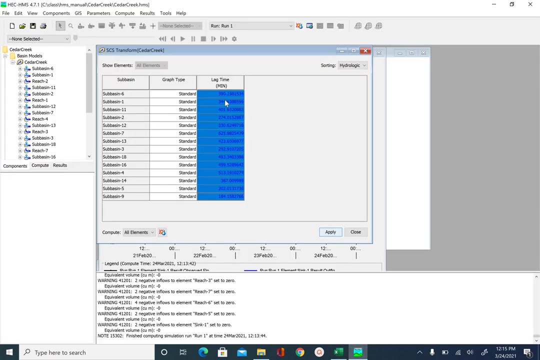 10 percent, 20 percent, pick your number, so i'm going to try 20 percent. so equal to 1.2 times the initial value, and do this for all and then copy these new values. ctrl c, and then we will paste it here. ctrl v apply. close and run the simulation again. 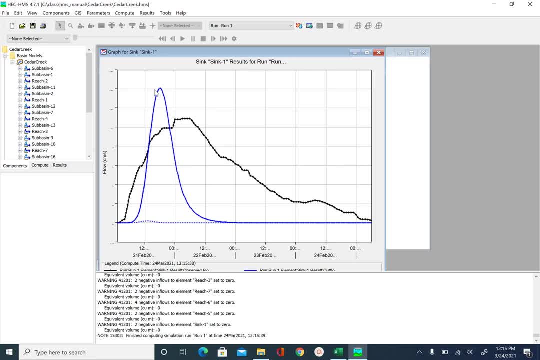 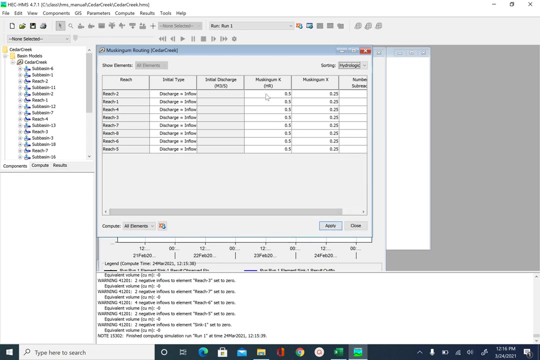 and you can see the peak came down a little bit, little more, and hopefully it also shifted towards the observed peak. so that is another parameter that we can play around. the third parameter that we can play around is related to routing. so we will go to routing muskingum so we can change k values. so this will affect the shape of the. 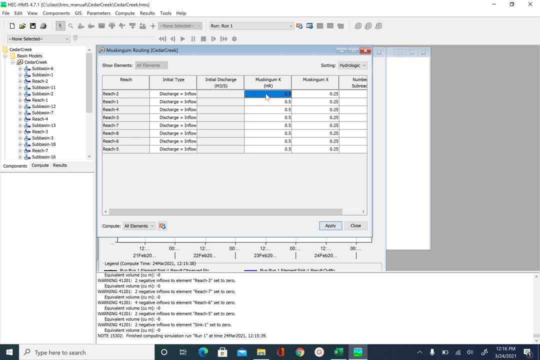 hydrograph also. so our initial value is 0.5. let's try to make it two or one, whichever. so this is a trial and error, iterative process, subjective process. so depending on which parameter value you pick and how many parameters you pick, you will get different results. 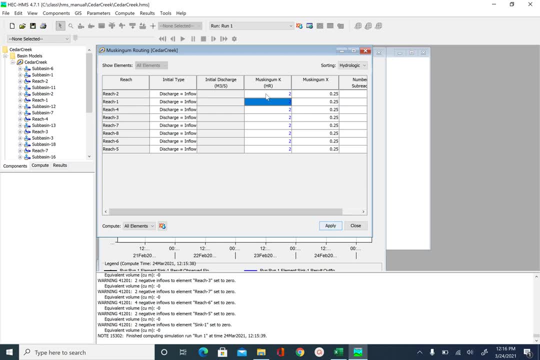 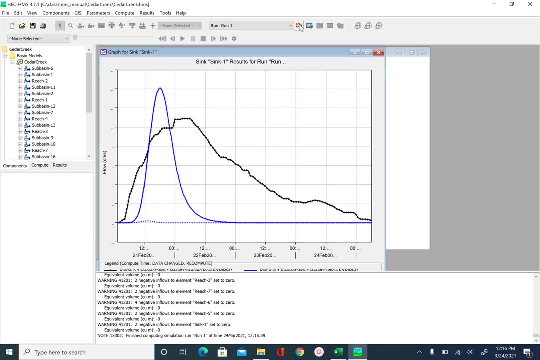 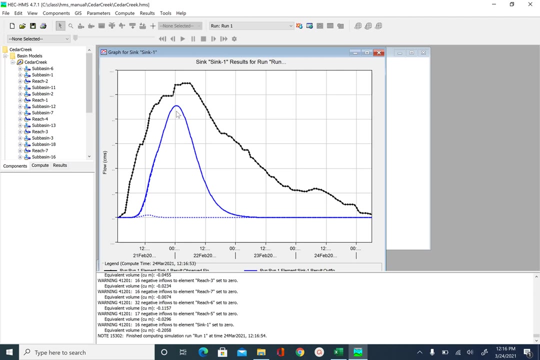 and many of us may get similar output with different parameter values. so we change k to 2, apply close and run again. and now you can see the peak came down significantly. now, if you want, you can increase the k value to 1, bring the peak little bit up and you may even have to go. 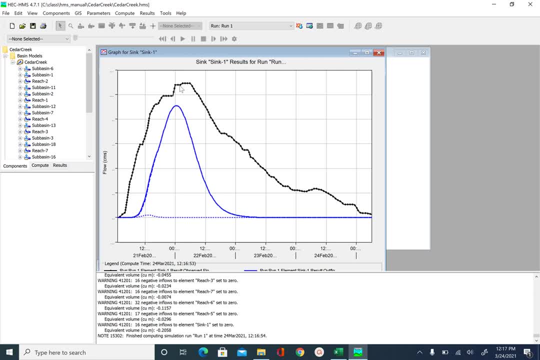 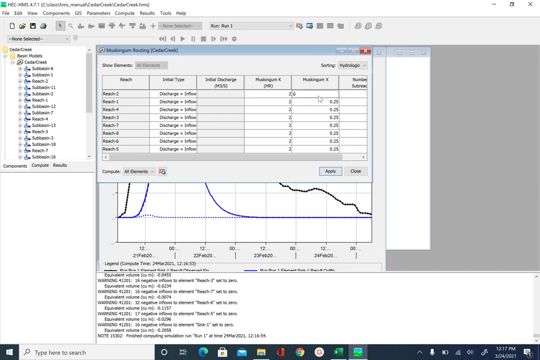 back to curve number and lag time and adjust that depending on your new k values. so let's go back and also look at how we can change x. so go to parameters, routing, and we can see that the peak is 0.25. so what if i make it 0.1? 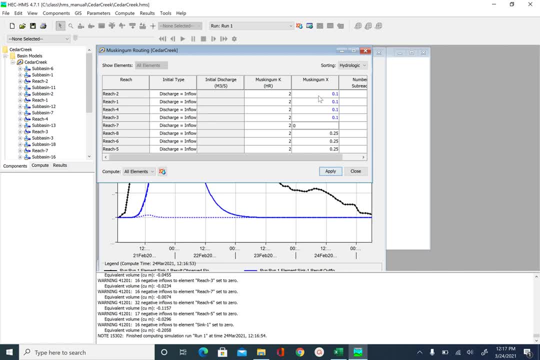 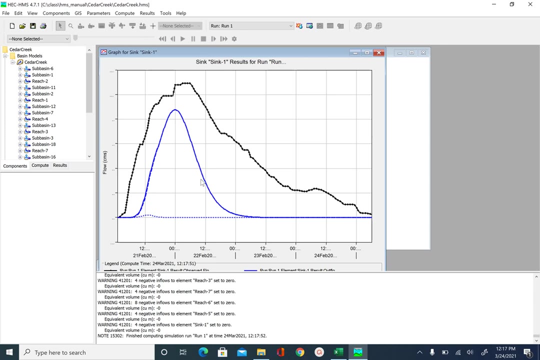 i'm not doing this in excel because we have only few values, so it is easier to do it here: apply, close and run again and you can see it has subtle effect, but not as significant as we saw with k, lag time and curve number. so in manual calibration you have to repeat this. 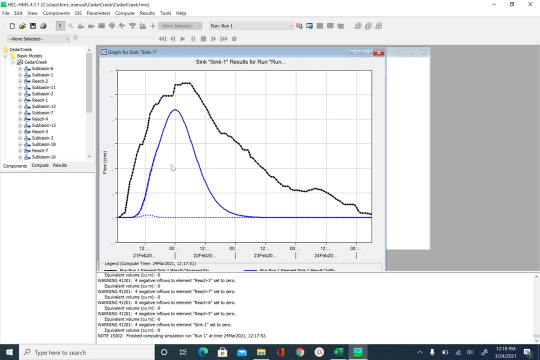 process iteratively, sometimes changing curve number, sometimes changing lag time, sometimes changing muskingum k and x to match the observed hydrograph with the simulated hydrograph. so right now we are just doing a visual comparison. so this is the result of the simulation and actually, as you get closer to observed, 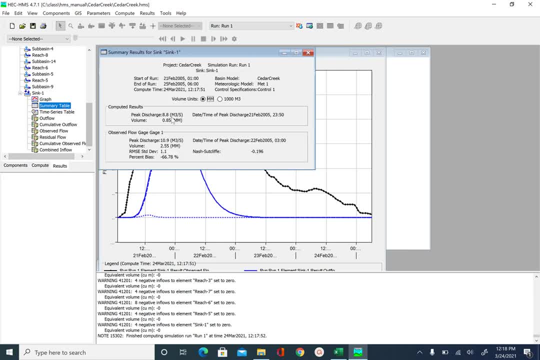 hydrograph. with your model simulation you can also look at other results, such as summary: how is the peak discharge matching? how is the volume matching? for observed and computed hydrograph, you can see the root mean square error: nash sutliff. so this should come close to 1 as these two hydrographs come together. 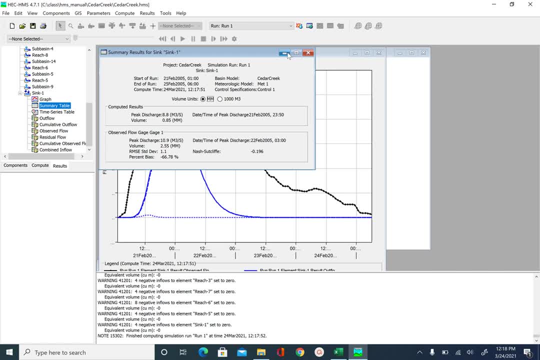 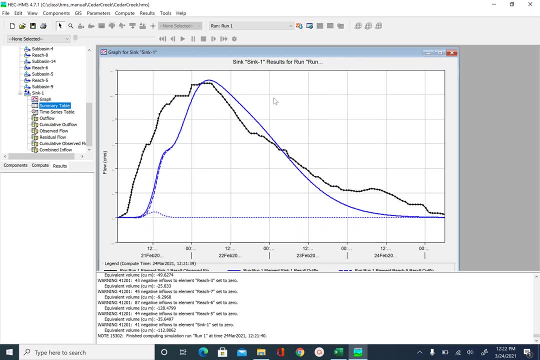 so this is the result of the simulation, and i just repeat this process until you get satisfactory output. so just keep working on it iteratively until you get satisfactory results, and i just want to show you the kind of improvement that you can expect from this manual calibration. so this is 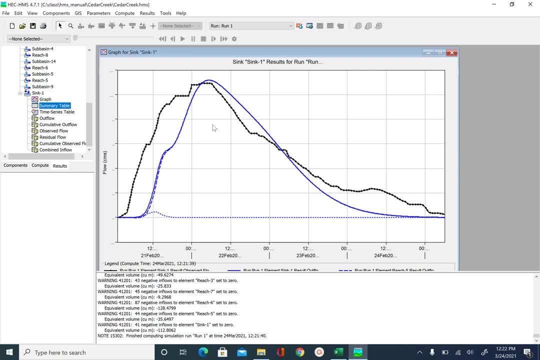 the output that i got after, say, 10 iterations of changing curve number, lag time, muskingum k and x. so you can see the peak and the peak time are matching okay. even the shape looks good. this is a little bit mismatched, but if you spend more time, 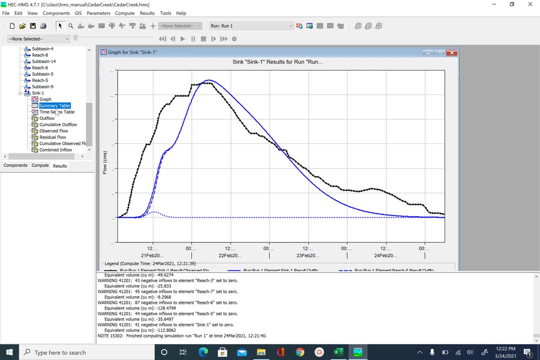 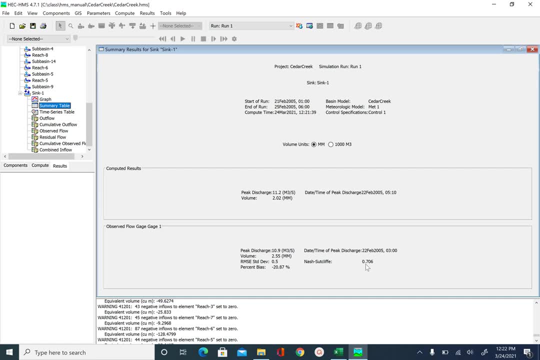 you should also be able to do that, and if i look at the summary table, you can see my nash sutliff is 0.7, which is pretty good. so our goal is to bring it as close to 1, and you saw in our first iteration this small course, Kara, which is a little bit like plasma. bye. laughing due to all the differences in copy copings i can't ThruPoint out your data's a powerful tool, which is pero. I used Bogsen and leave no lag to R, of which all these methods you can see in the currentハnガ Informationen.